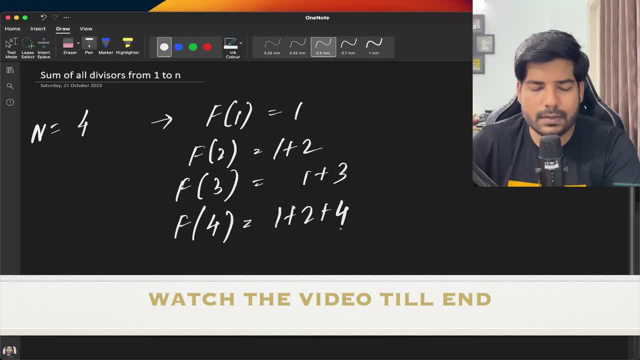 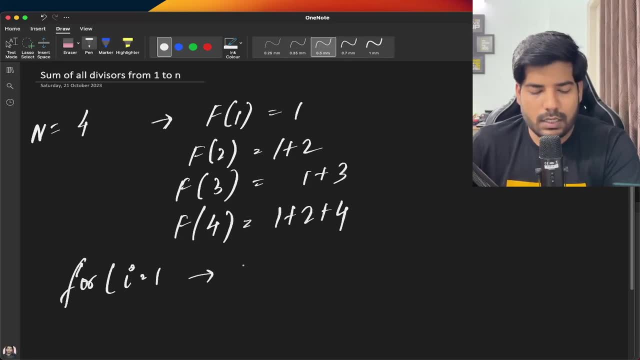 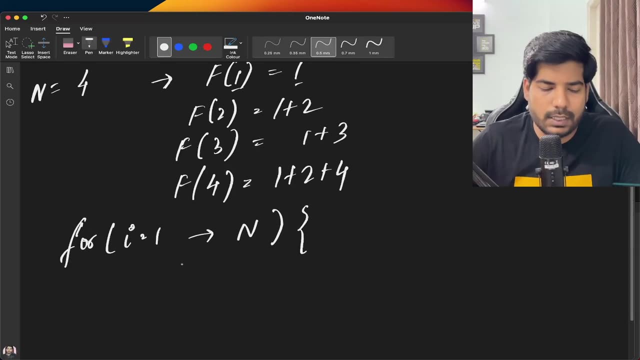 is going to be 1 plus 2 plus 4 right Now. the brute force approach is that you just simply run a loop for i equal to 1 till i less than equal to n. okay, because we need to find the divisors for all numbers from 1 to n. 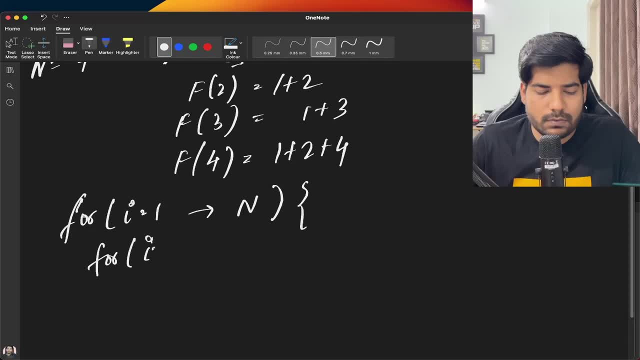 Now you can simply run a loop inside this for int, j equal to 1, j less than equal to i and j plus plus. So let's say, for i is 1, you will run your loop from 1 to 1 and you will check if i is. 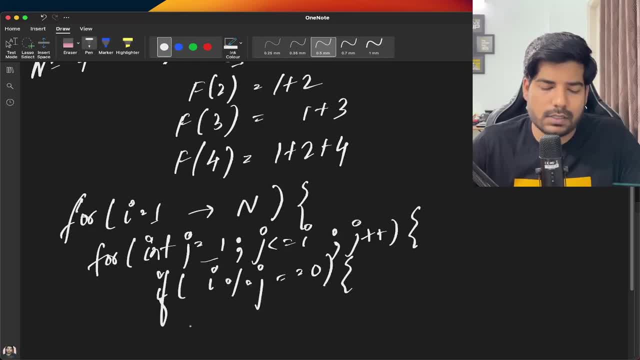 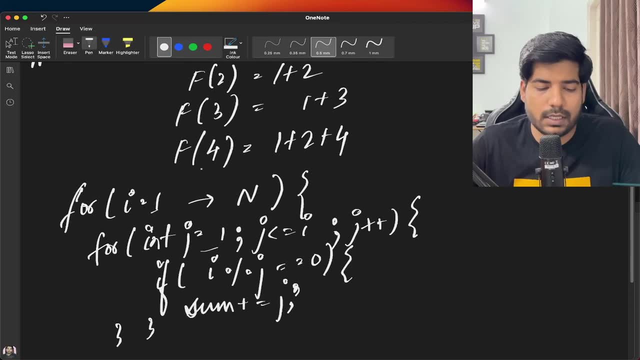 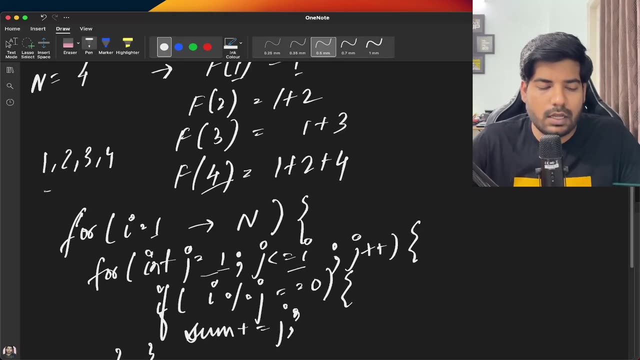 divisible by j or not. If it is divisible, you will simply sum up j into your variable sum and you can get your answer right, For your j will run from 1 to 4 and you will check for each of the values, basically 1, 2, 3, 4 and. 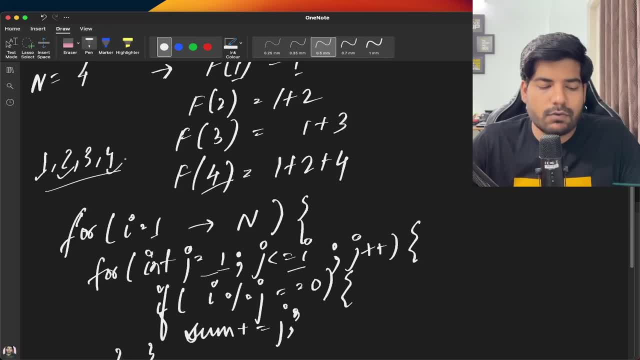 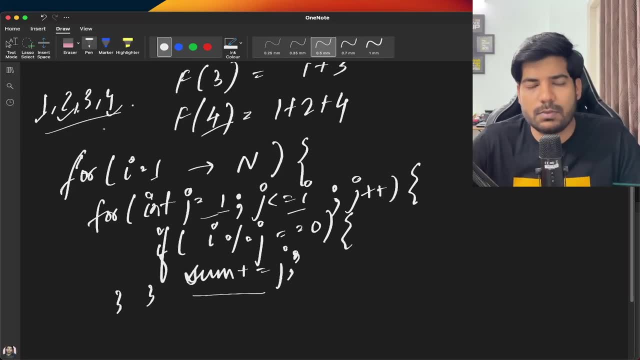 1 will divide 4, 2 will divide 4 and 4 will divide 4.. So here you will add up 7 here, okay, because 1 plus 2 plus 4 is going to be nothing but 7 and in the end you can get your answer. But in this. 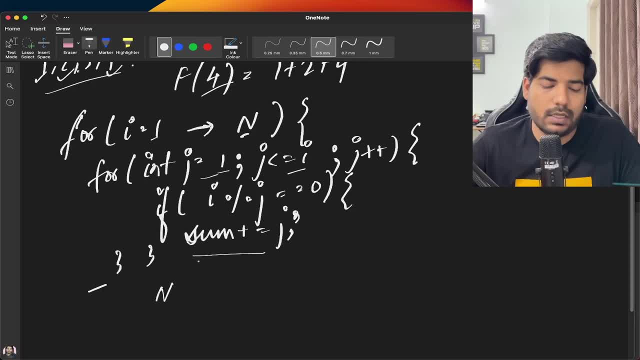 approach your i can be maximum up to n and j can be less than equal to i. So j, in worst case, will be equal to n. This will be an order of n. square time complexity, The space complexity here will be nothing but order of 1, right, because you are simply using a sum variable. Now one solution will come to your. 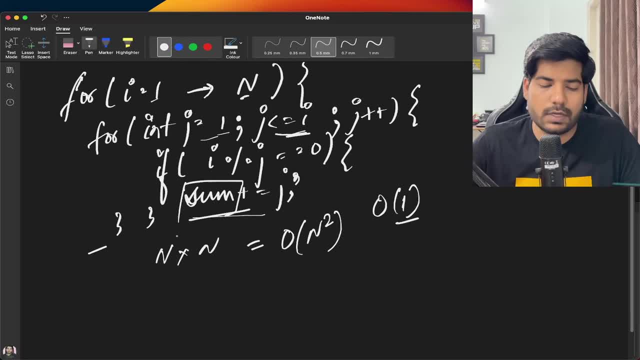 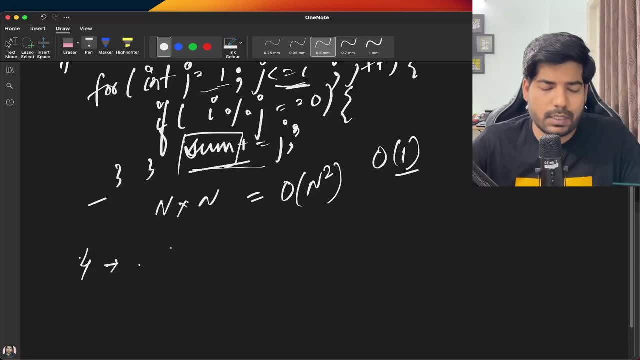 mind, Let's run this j till square root of i, So you can do that as well. Basically, if you observe any number, let's say 4, 4's multiples are going to be nothing but 1 into 4, 2 into 2 and 4 into. 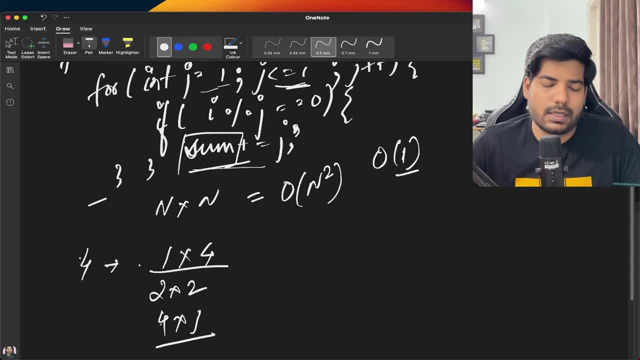 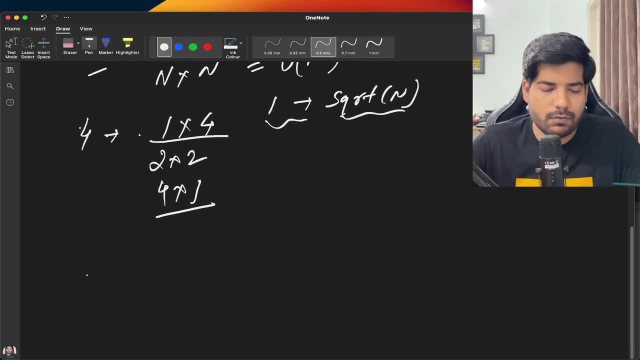 1.. So these and these are repeating, right? So what we can do? we can simply run our loop from 1 to square root of a given number, n, and we can calculate all the factors, right? So how can we do that? Basically, for 4, we will run our loop for j equal to 1 till j less than equal to square root of 4. 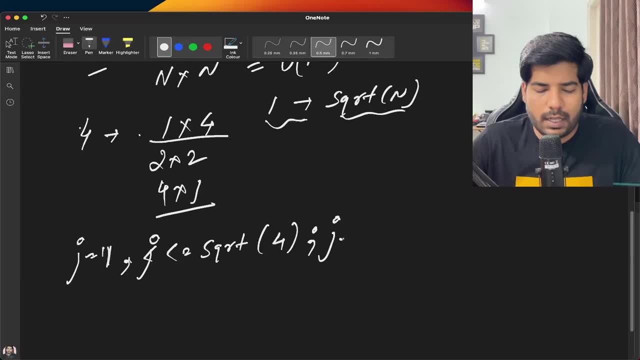 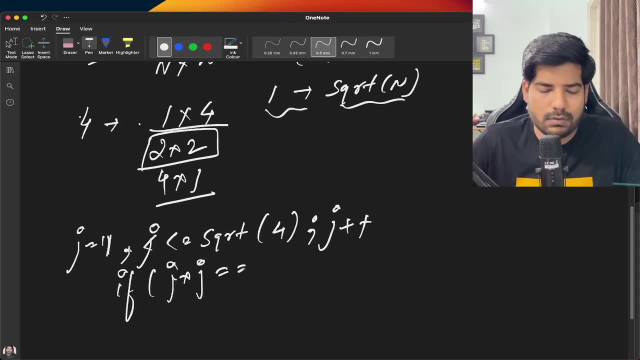 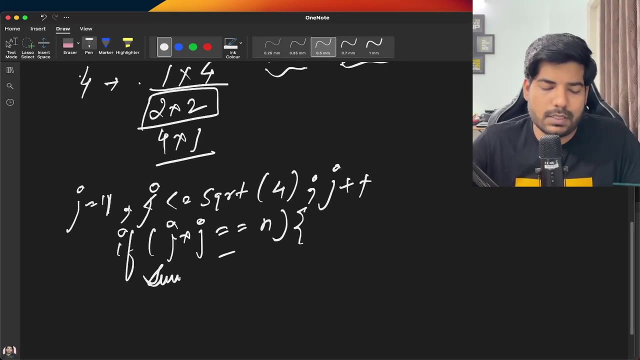 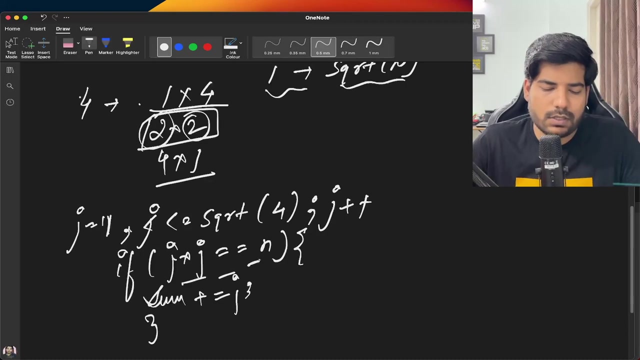 which is 2.. And you will simply check if, basically, j into j is equal to n, right? so that is a corner case for a perfect square numbers. in this case, you will be simply summing up j in your answer. otherwise you know like, for example, if j into j is equal. 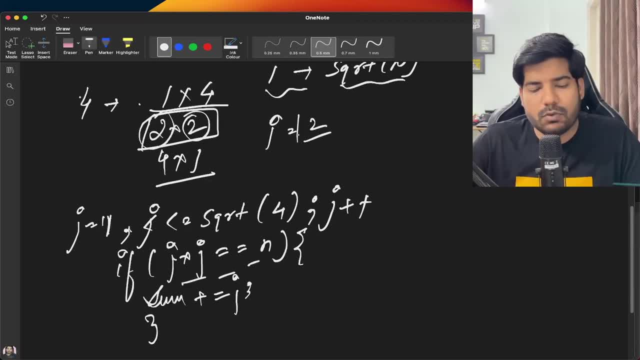 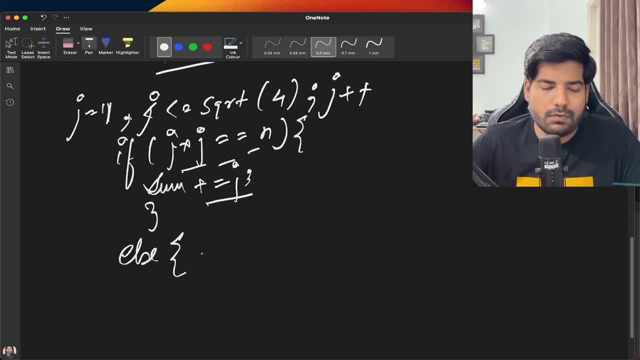 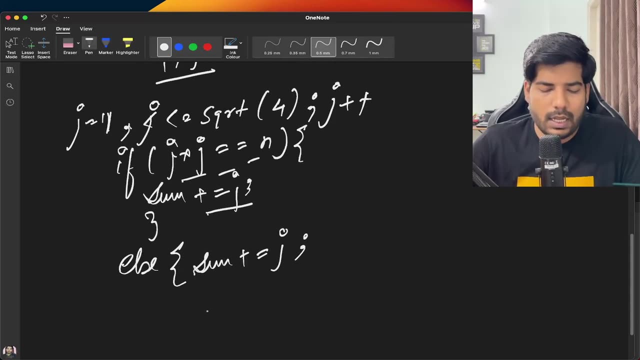 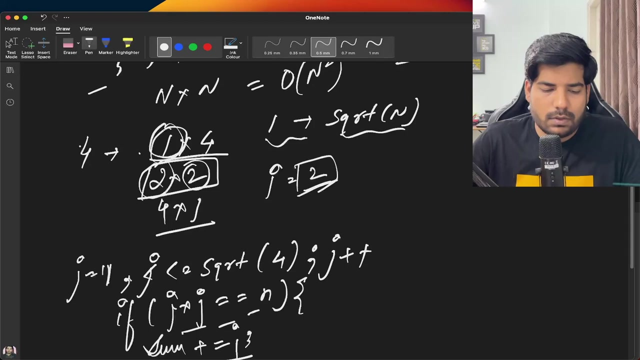 to n means your j is going to be 2, so will you add up to twice? no, you will add up to only once, right? otherwise you will end up adding 1, right? so that will be nothing but j and your other number is going to be nothing but i by j. okay, so j is going to be 1 initially. your other number is: 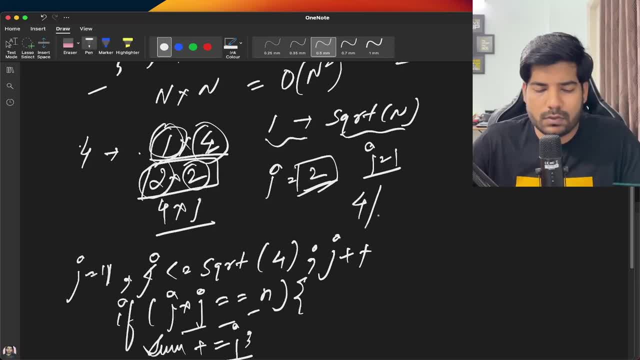 going to be nothing. but let's say i was 4, so 4 divided by j, which is equal to 4 itself. so you will add up 1. you will add up 4 here. when you are at this case, you will add up two, only ones, so your overall sum will be: 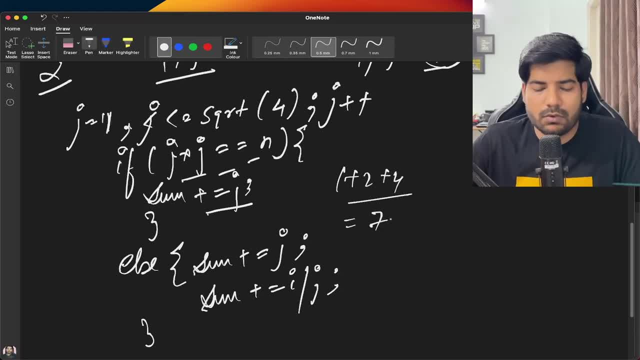 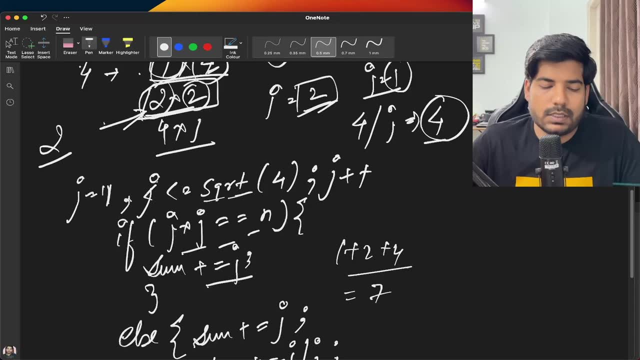 nothing but 1 plus 2 plus 4, which is expected, which is equal to 7 right now. what will be the time complexity for this approach? here you are using j loop, which is running from 1 to square root of n, so that you have optimized your time complexity to root n, but your outer loop i will 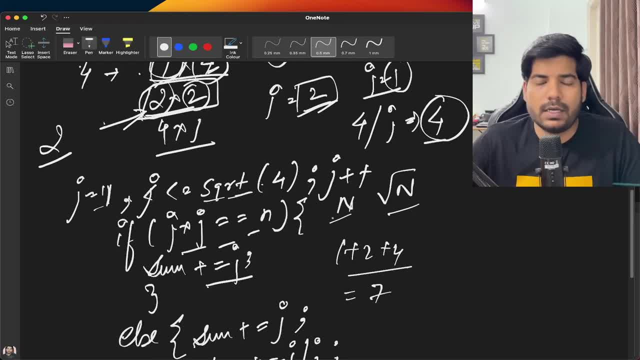 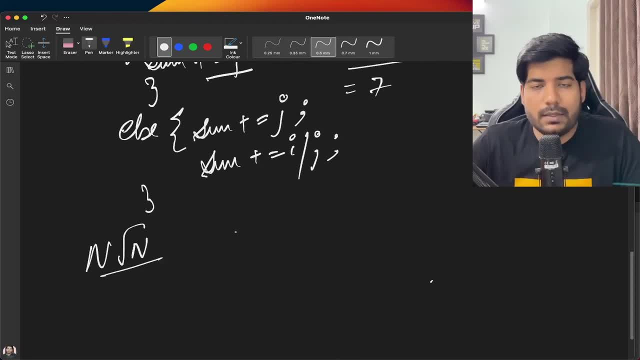 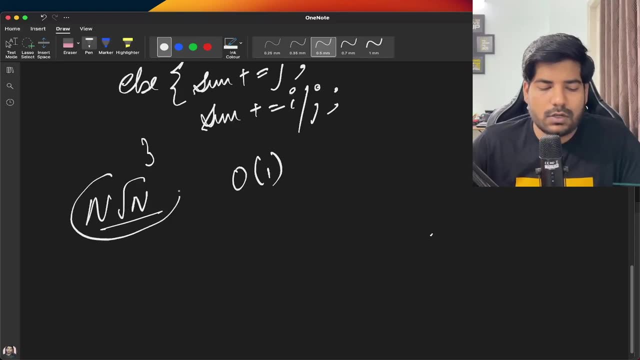 be running for n times, because you need to do this for every numbers from 1 to n, so your overall time complexity will be nothing but n, root n, and your space complexity here will also be order of 1. okay, now, this will not solve our purpose, because n can be up to the range of 10 to the power 6. 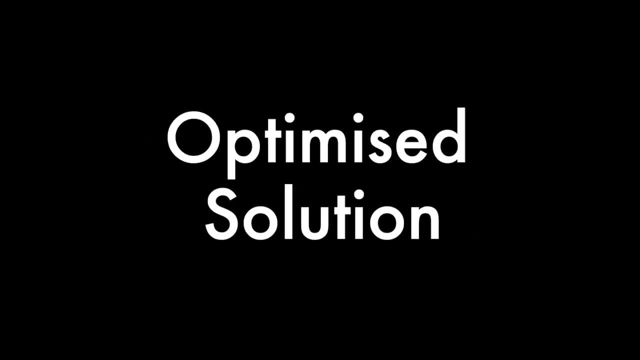 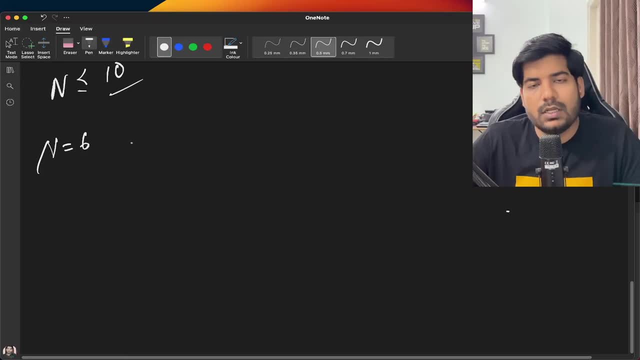 now we need to further optimize it. so, if you carefully observe the pattern, let's say our n n is going to be 6. okay, so we need to calculate the sum of all the devices for every n from 1 to 6. okay, so let's write it so: f of 1 is going to be 1, f of 2 is also going to be 1 plus 2. f of 3 is going: 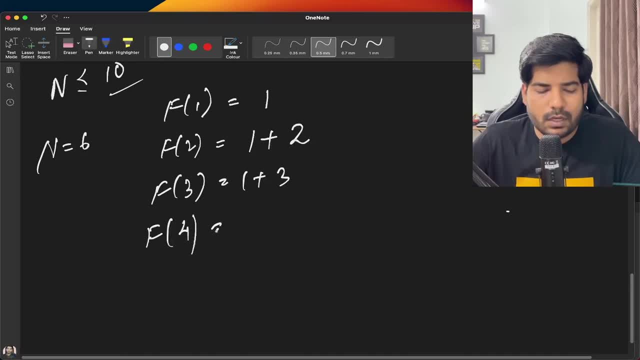 to be 1 plus 3, f of 4 is going to be 1 plus 2 plus 4, f of 5 is going to be 1 plus 5 and f of 6 is going to be 1 plus 2 plus 3. 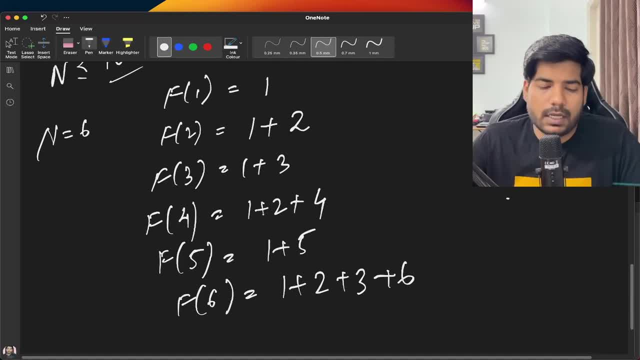 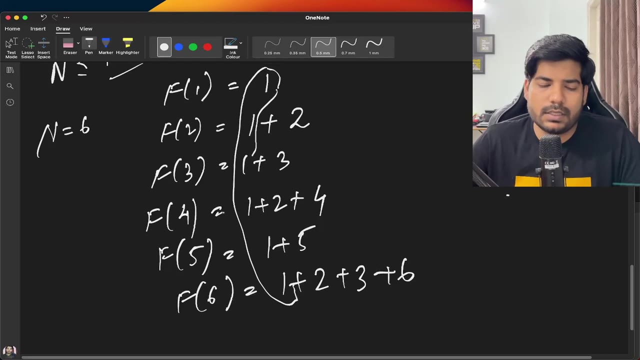 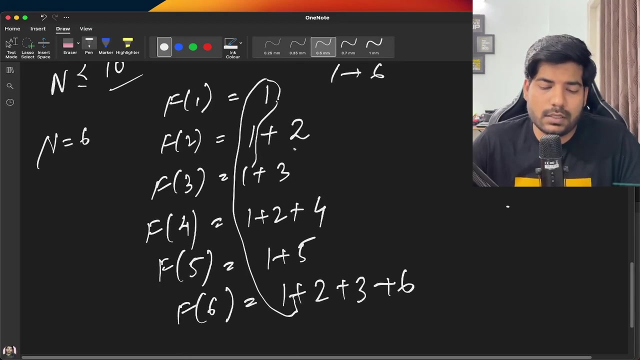 plus 6. now you can observe one thing here, like in this: overall how much times one has occurred? one has occurred nothing but six times, right, because you know one is the factor for every number. so one has occurred six times. right now, how much time two has occurred. two has occurred. 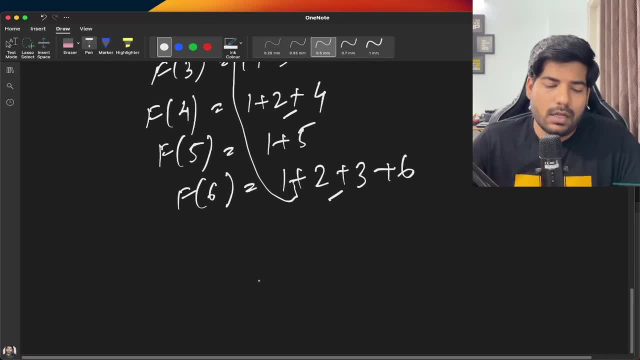 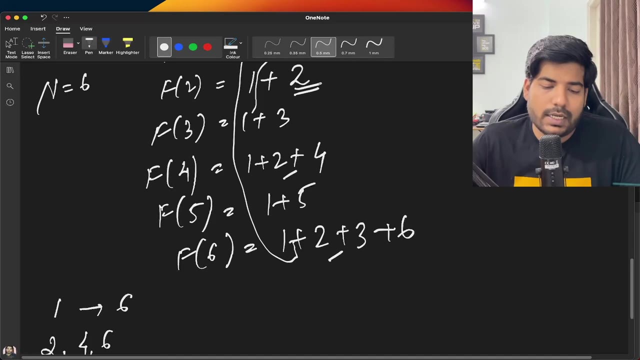 here. two has occurred here and two has occurred here now. if you observe the pattern you can see here: two has occurred here and two has occurred here now. if you observe from one to six, what are all the numbers which divides two? basically two, four and six right and two has occurred thrice as well. 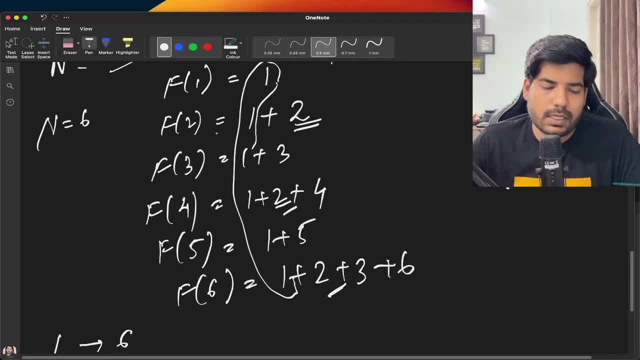 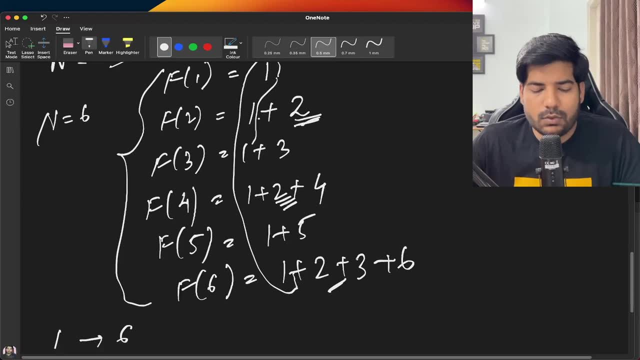 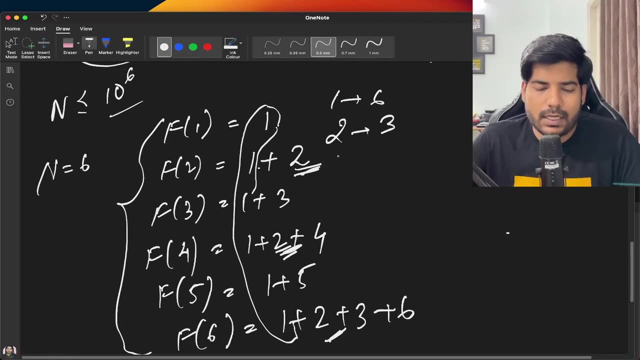 so you observed one thing basically here, from here to here, whatever number we have, okay, whatever is being divided by two at the same time, two is also occurring in this pattern, right? so two is occurring. 2 has occurred 3 times. Similarly, how many times 3 has occurred? 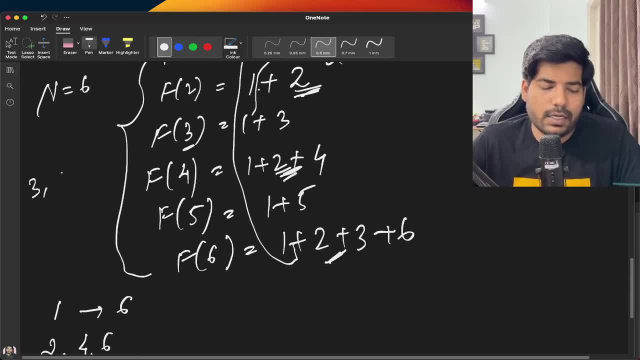 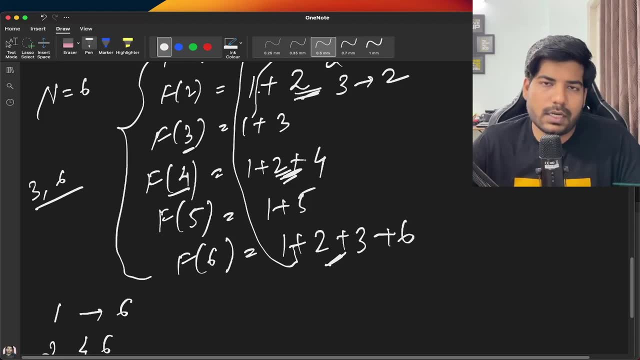 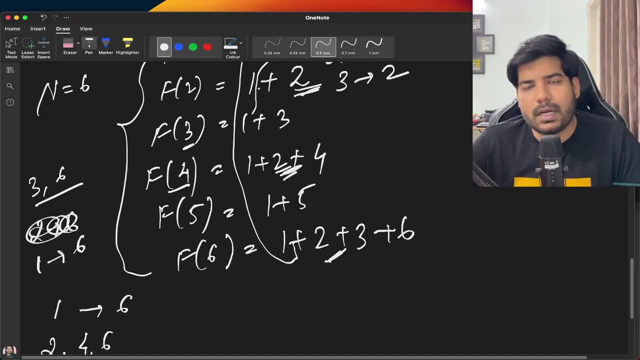 3 has occurred in 1 to 6.. It divides 3 and 6.. So 3 has occurred 2 times, Right? Similarly, how many times 4 has occurred From 2 to 6.. Sorry, From 1 to 6, 4 has only divided 4. Right. 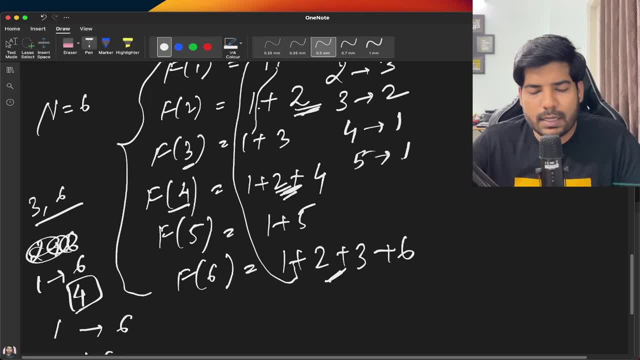 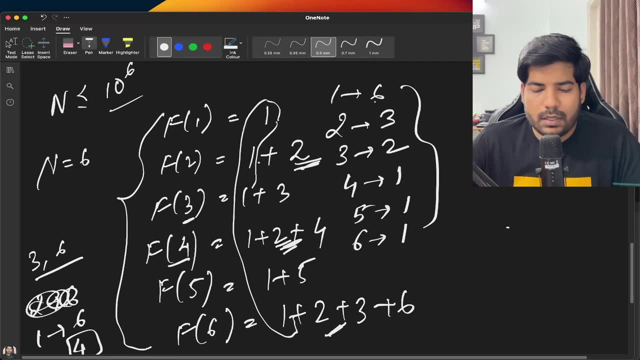 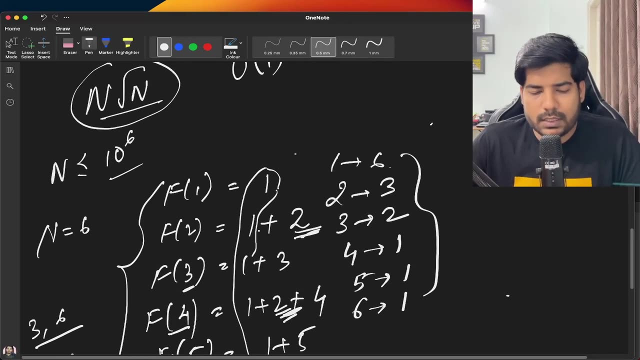 So 4 has occurred 1 time. Similarly, 5 has occurred 1 time and 6 has occurred 1 time. Now, what you can do, You can simply multiply them, Okay? So here 1 has occurred 6 times. 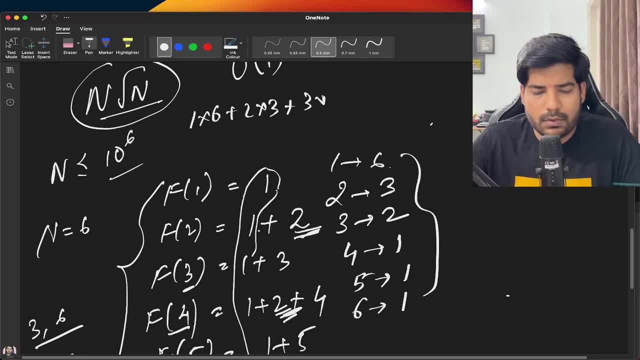 So 1 into 6 plus 2 into 3 plus 3, into 2 plus 4 plus 5 plus 6.. Right, So this is going to be 6.. This is going to be again 6.. This is again going to be 6.. 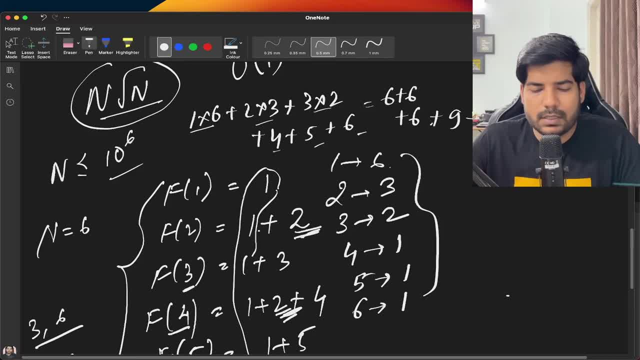 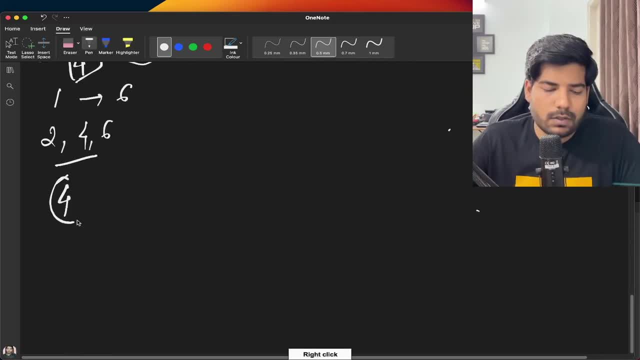 This is 4 plus 5 plus 6.. So 9 plus 6.. Right, So this is going to be 24 plus 9, 33.. Now, similarly, if you observe, for 4.. So for 4, f of 1 is going to be 1.. 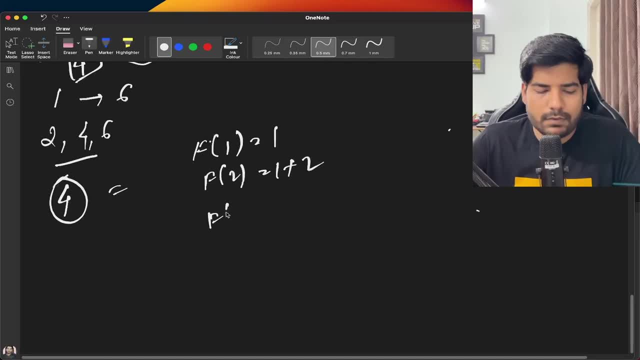 f of 2 is going to be 1 plus 2.. f of 3 is again going to be 1 plus 3.. And f of 4 is going to be 1 plus 2 plus 4.. For n equal to 4, our answer was 15.. 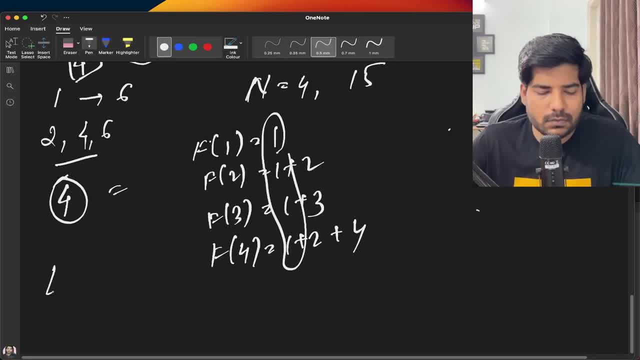 So 1 has occurred 4 times. So let's add up 4.. 2 has occurred 2 times. So 2 into 2 plus 3 has occurred 1 times, plus 4 has occurred 1 times. 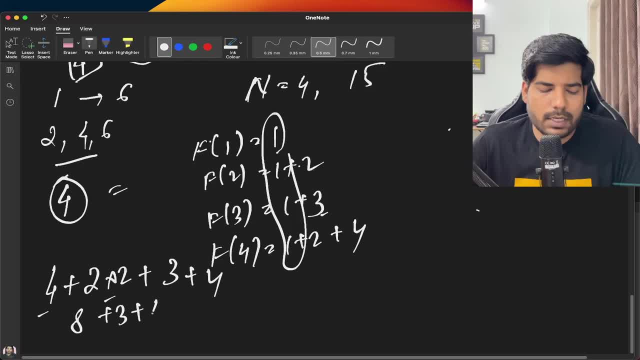 So 4 plus 4 is going to be 8, plus 3 is going to be 11 plus 4 is going to be 15.. So in this way, you can get your answer Now. in order to get this, what you will be doing, 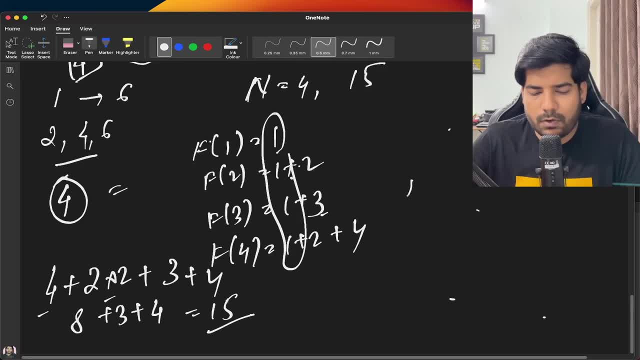 Like you will be simply running a for loop for i equal to 1 to n. Right Now, your 1 will be occurring. Your 1 will be occurring. how much times It will be occurring? nothing but n by i times, Right. 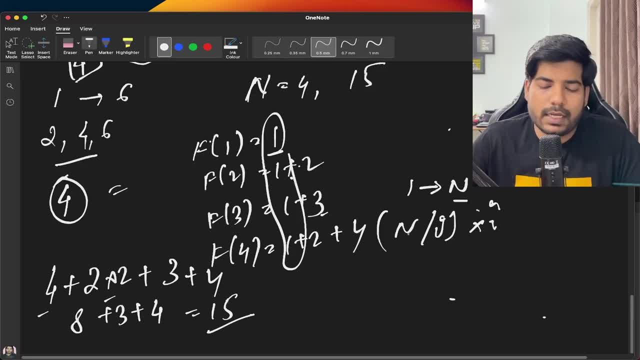 And you will simply multiply this by i, because your i here is going to be 1 for the first loop. So you will simply add up i into n by i to your answer And you can run your loop from 1 to n. 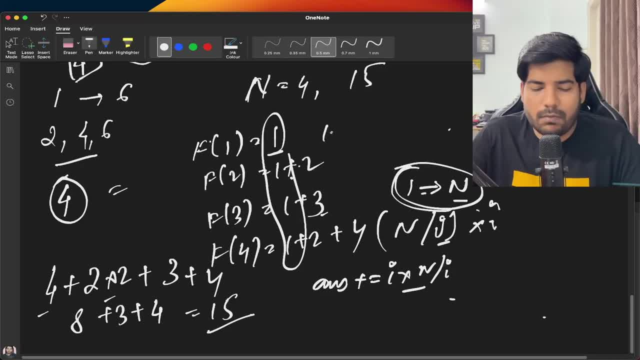 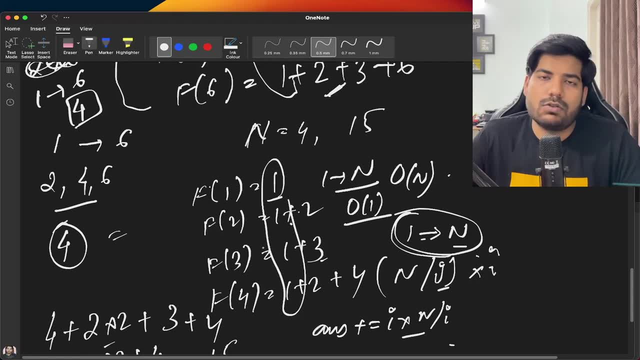 In this way, your loop will be running from 1 to n And it will be taking order of n times And your space complexity will also be order of 1.. So I hope you have understood the problem. Let's discuss the implementation. 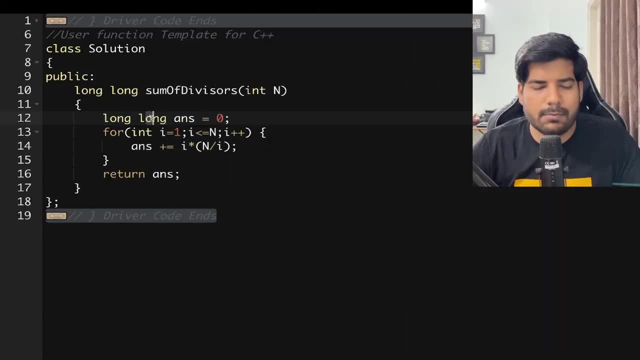 First of all, we have taken a variable answer which is of type long, long Okay, And we will be simply running a loop from i equal to 1 till i less than equal to n, Because we need to do the operations for every numbers from 1 to n. 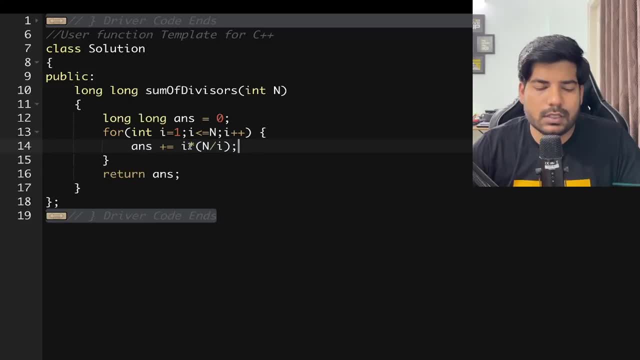 And we will be simply adding up i into n by i, because, let's say, i is my current number And it will occur n by i from 1 to n, Right As we discussed, And we will add it up And we can simply return our answer.